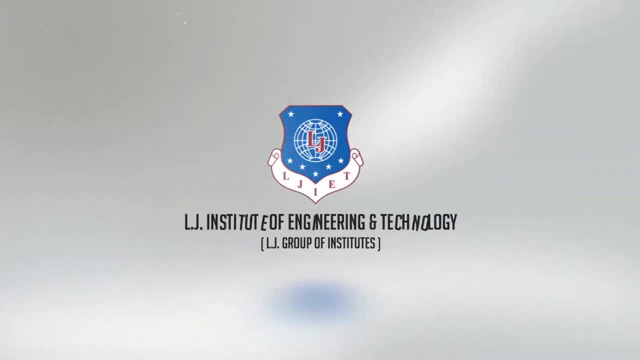 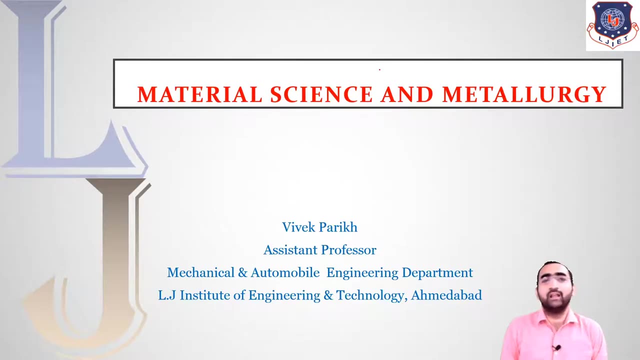 Hello everyone, welcome back to the online sessions of the material science and metallurgy Myself, Vivek Parikh. we are going to discuss about the crystal structure and crystal geometry. in this lecture We have already gone through the things that: what is the unit cell? what 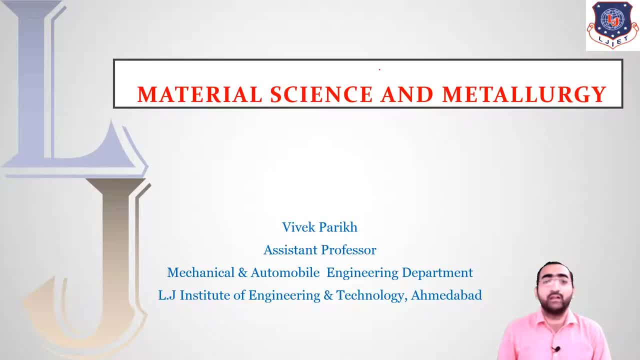 are the different types of the atomic packing factor. we have gone for the derivation, then we have gone how they are increasing, the direction, the plane that we have studied, Miller indices: we have gone through. So about the crystal, we have studied. Now there are 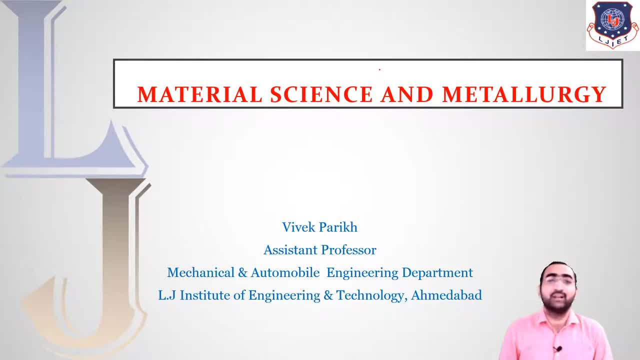 always a chances of the defects which are occurring inside the crystal. So how many types of the defects which are likely to occur in the crystal? so that thing that means the imperfection of the crystals, that thing we will be discussing in our today's lecture. 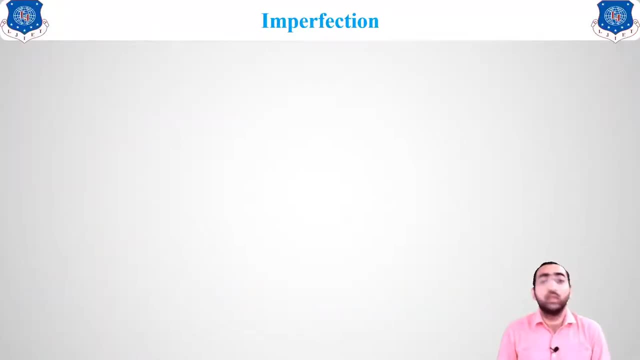 So let us start with the topic that is known as an imperfection. Now, what do you mean by imperfection? That is basically, it is the study which indicates the defects which are there inside the material. So that means, in a crystal, which are the chances, or which are the likely chances of the defects? 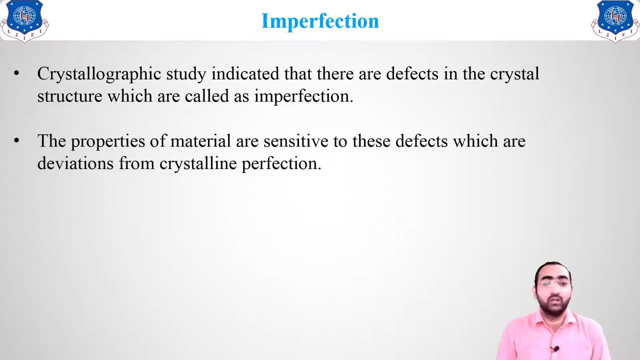 to get inside the particular crystal structure. So the properties of the material, as you know, they are very much sensitive. So if there is any of the defect which is occurring inside the particular crystal system then there are likely chances the properties of the material will always get deteriorated. 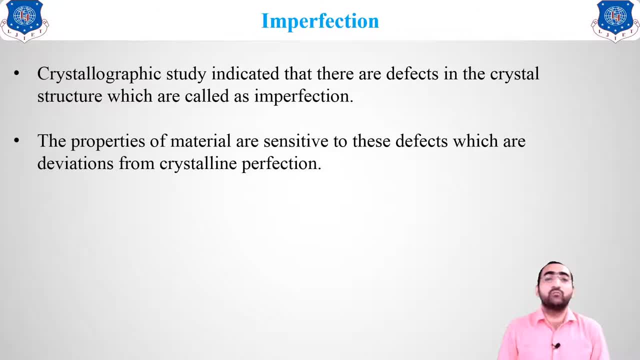 So that is the reason why we have to go or we have to study about this particular imperfection. The effect of this defect is always- not always- adverse. Why? Because sometimes there are also. it is helpful for us for getting certain types of the properties. As I give you an example: we are adding an impurity like a copper in. 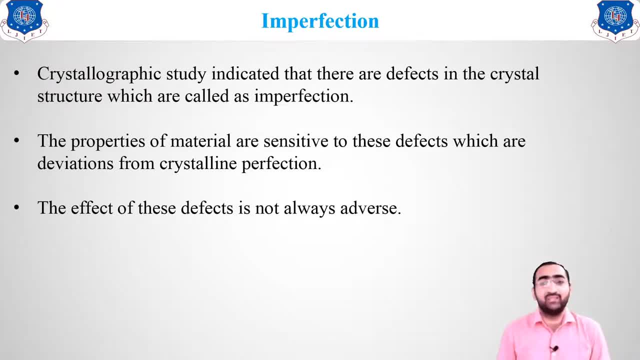 a gold, so that the strength of the gold is increased. So in this way, if you insert any of the impurities inside the material, then also it will get deteriorated. So that is the reason why we have to go or we have to study about this particular imperfection. 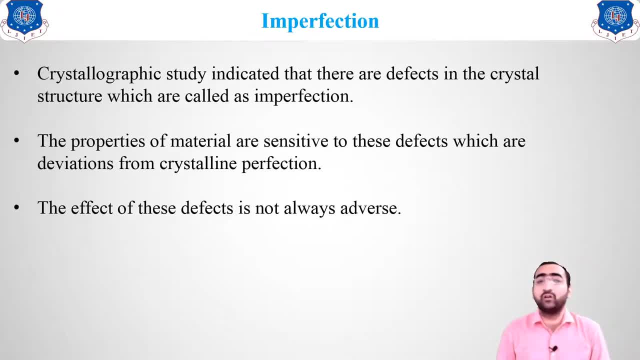 is helpful for us. that means the imperfection. they are not always giving you the adverse effect. they are always having a both the side adverse, majorly adverse. but sometimes they also gives us the beneficiary thing. that means this is how the imperfection works. so sometimes of the certain 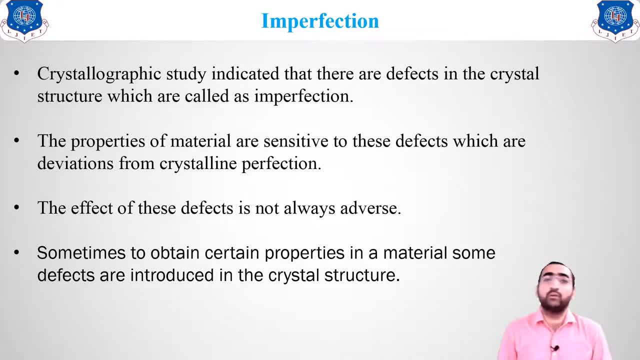 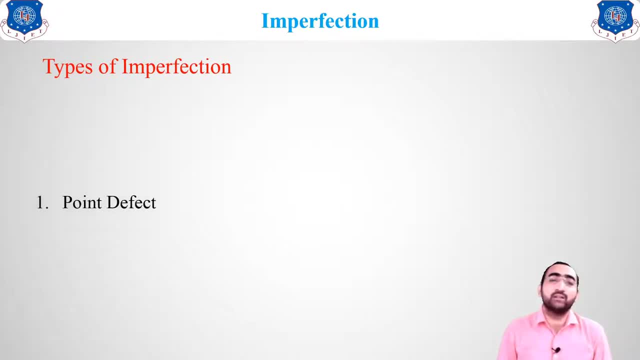 properties of the material defect. sometimes they increase the properties and sometimes they will decrease the properties. so how many types of the defects are there? types of the imperfection, they are the point defect which is affected by a certain single atom, or linear defect, in that the whole line of atoms they are creating the defect. then surface defect: the whole surface. 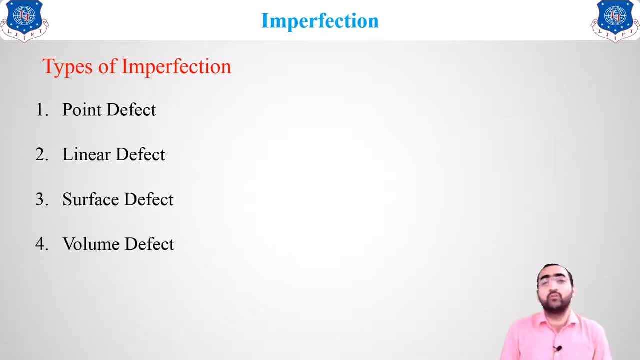 is having a problem, and the last one that is known as a volume defect. so in today's lecture we will discuss all this type of the defects which are occurring inside the material. so let us start with the first one, that is the point defect. it is attached by the movement of only 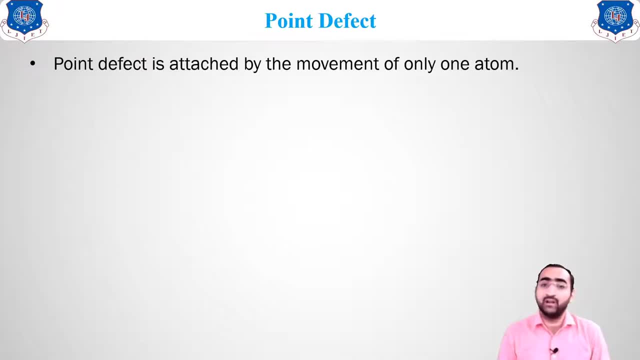 one atom, that means with the help of or only one atom is responsible for the defect. all atom possess vibrational. when they are at the stationary thing, when the crystal is in position, what will happen? the atoms will constantly vibrate and when this vibrational energy exceeds certain limit, the atom breaks. 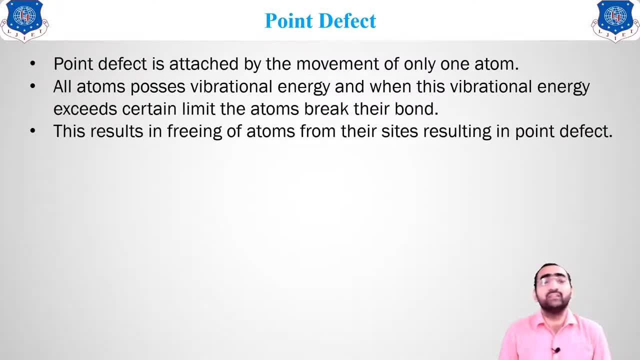 the bond and goes away. the result of freeing the atom will gives you a defect. point defect will occur, different types of point defects which are occurring. they are: vacancy defect, self interstitial defect, interstitial impurity defect, substitutional impurity defects, Schottky and the 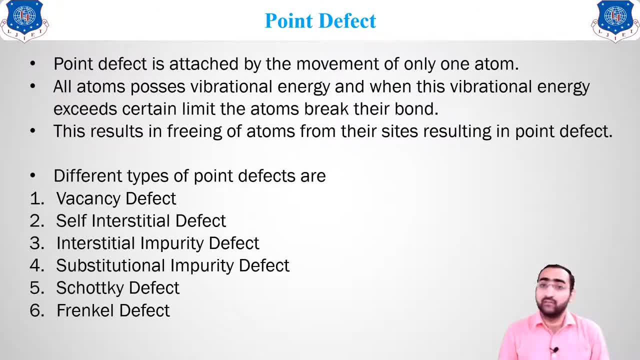 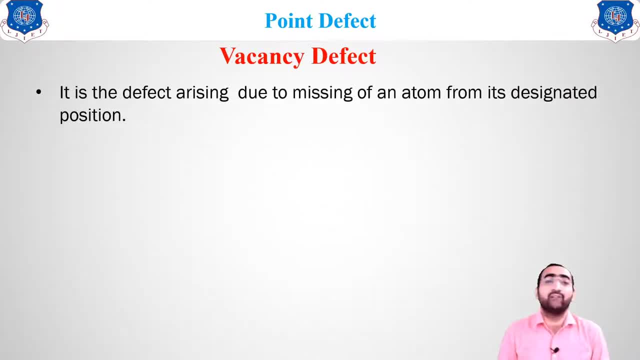 last one, Frank. also, there are six different types of the defects which are occurring inside the material, starting with the first one of weapons. a defect. weapons a defect. it is the defect why arising when a single atom leaves its position and goes away, the defect which is generated inside a 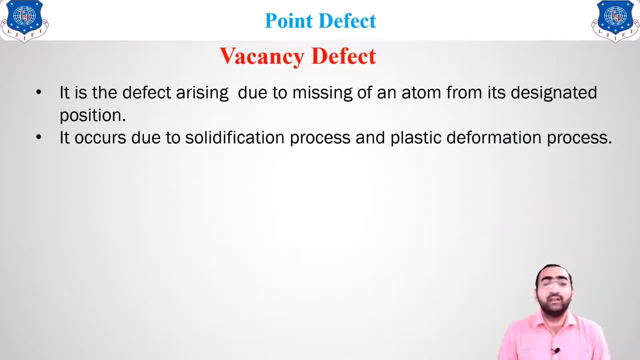 crystal that is known as an vacancy defect. why it occurs? it occurs due to solidification process or the plastic deformation process. it occurs due to this two major reason: almost all the crystalline they are having some other another vacancy defect is always present in all, each and every crystals. this is the type of the thing, how it looks this one atom has. 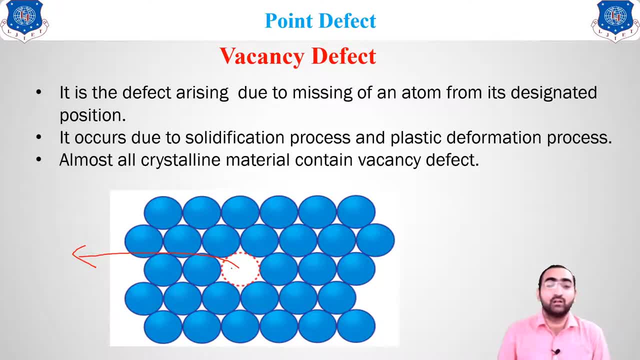 gone away from its original site and leaving the whole, or you can say a vacant space inside that thing. that's why it is known as an vacancy defect, clear going with the second one. the second one that is known as an self-interstitial defect, when an atom leaves. 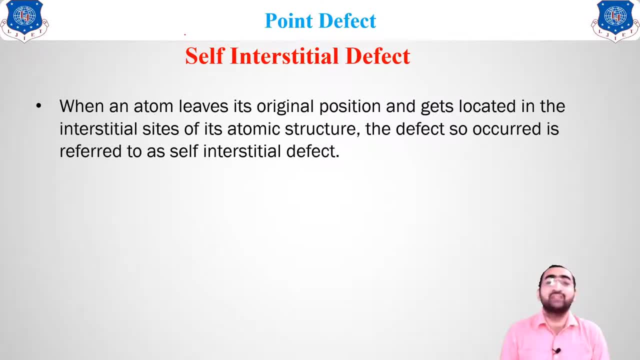 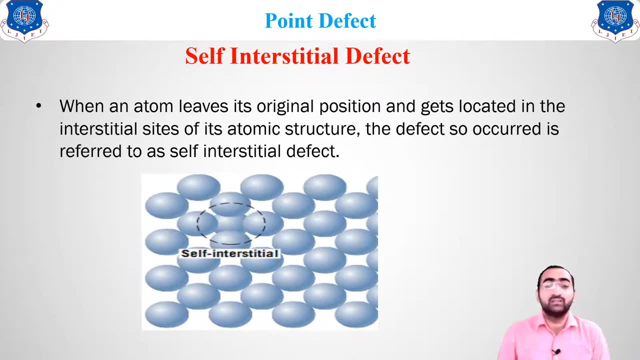 its original position and get located in the sides of the atomic structure. the defect which is occurring, that is known as a self-interstitial. you can see over here this is a self-interstitial defect, how this atom, this atom from any other sources have gone and settled over here in between. 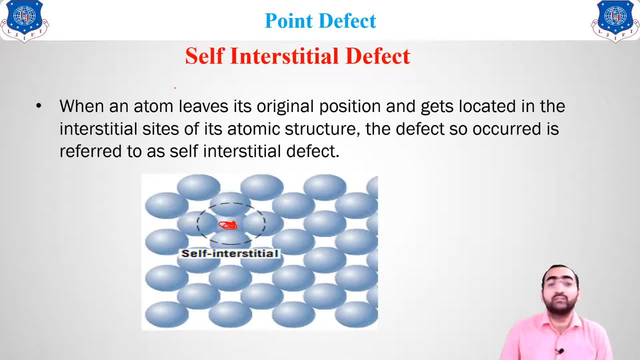 the particular atom, then this type of the defect is known as an self-interstitial defect. you have to see that the atom which is replaced or which is sitting at this area it is of the same size f of all these atoms. only so that is known as an self-interstitial defect. 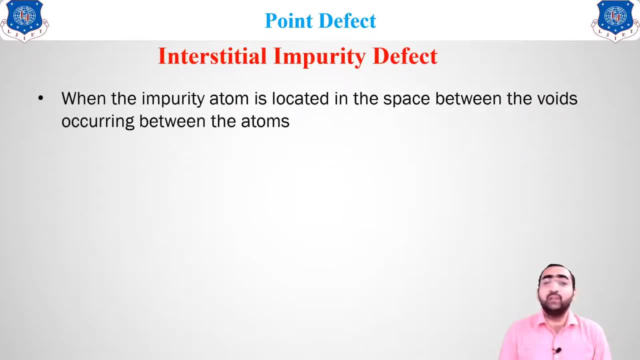 clear. then there is another interstitial impurity. when an impurity atom is located in the space between the atom, then that is known as an interstitial impurity. here the the, the thing which is going to settle over the space which is left between the atoms. larger atom, the. 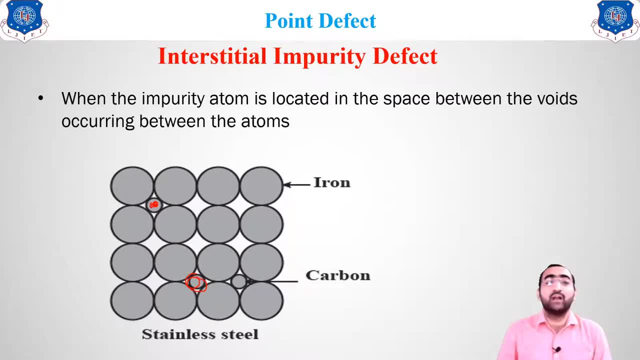 thing, which is impurities, will be going in the space which is left behind it. so that is known as an interstitial imperative defect. i told you, in a self-interstitial the size will remain same, but in an interstitial impurity, size of the impurity is very much small and they are located. 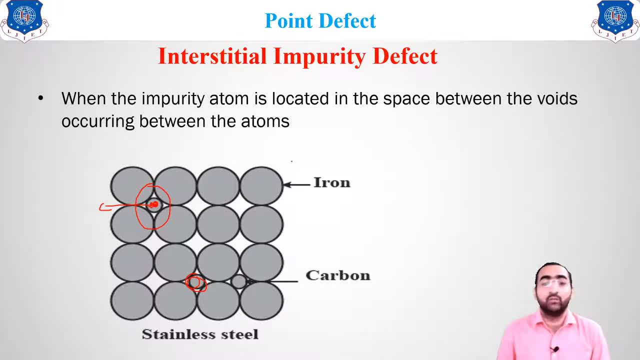 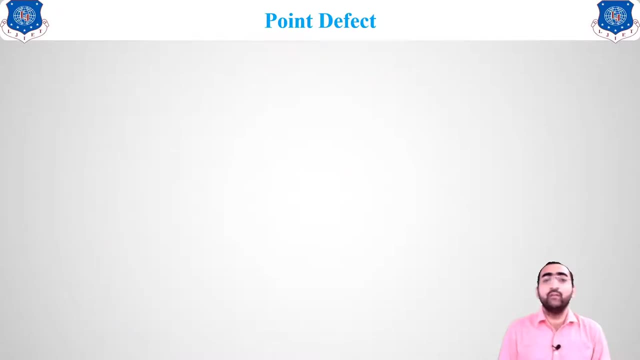 in the spaces which is left between the larger atom. this is the example of a stainless steel. iron is there? carbon is there? carbon is an impurity and it will settle down in the space which is left by the iron atoms clear. so that is your interstitial impurity defect, moving forward for the next one. 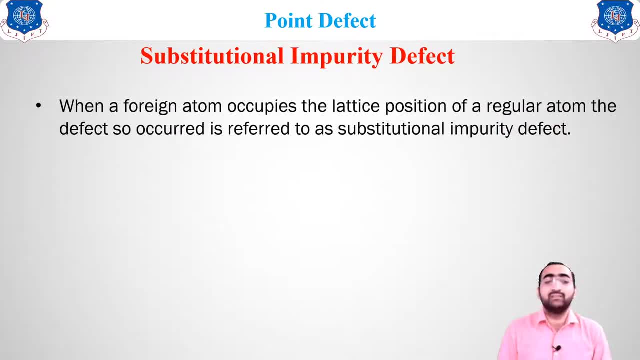 that is known as an substitutional imperative defect. what is this? substitutional impurity when a foreign atom occupies the latai space of the regular atom means whatever. any regular atom goes away and it has been replaced by any another foreign particle of the same size. that is the 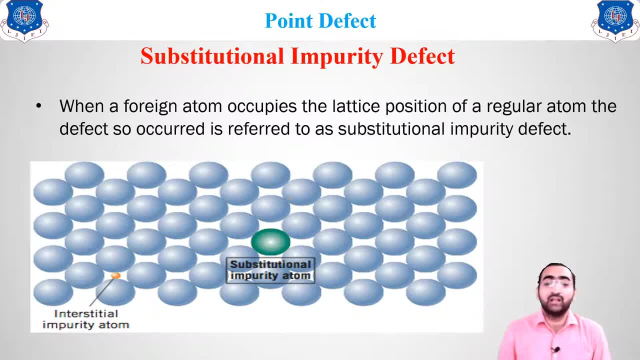 known as an substitutional imperative defect. these are the blue atoms which are there, but here one blue atom has gone away and one another thing that has come inside, that is known as an substitutional, of the same size green atom has replaced one blue atom that is known as. 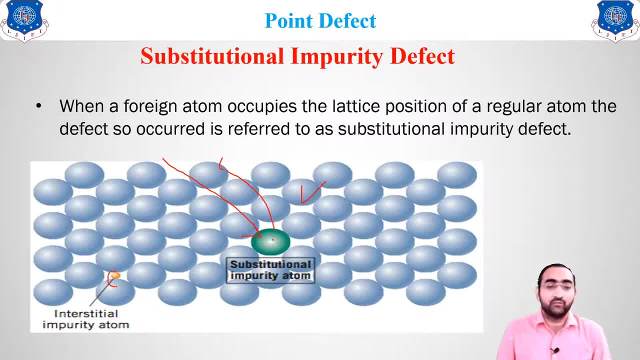 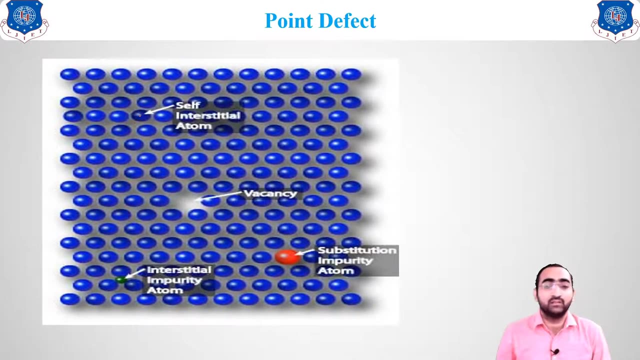 an substitutional impurity defect. if it is of the small size, it is interstitial impurity, and if the same atom is sitting in over here, then that is known as an self interstitial defect. let us see all this thing in this one thing. this is our self. 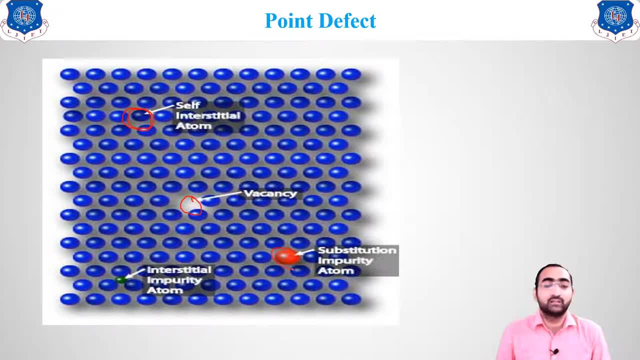 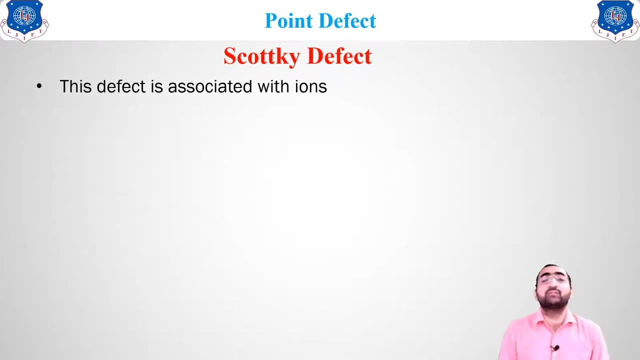 interstitial defect, vacancy defect, substitutional and interstitial clear. so these are the four defects which are there due to the atom. now, according to the ions, two defects are there. they are the short key defect. short key defect. they are associated with iron when a pair of 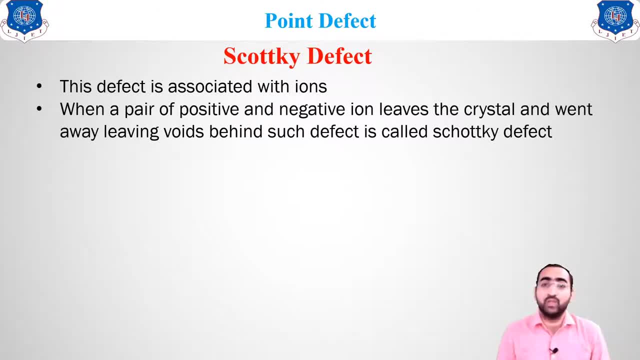 positive and a negative ion leaves the space of the crystal and goes away from the crystal, leaving behind the space, vacant space behind it, then that type of the defect is known as an short key defect. you can see over here: this is a perfect crystal plus minus, plus minus anion cation is there. but in this short key defect over here, one positive. 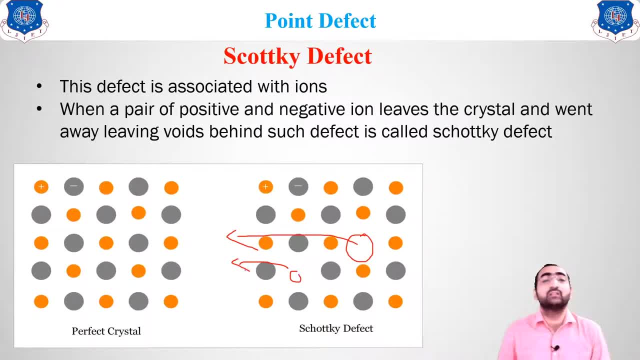 one negative ion has leave its space and just goes away, leaving behind the vacancy after the vacant space remaining in the crystal and creating a defect. this type of the defect where a one anion and one cation leaves the position of it and goes away. that is known as a short key defect. and the last point: 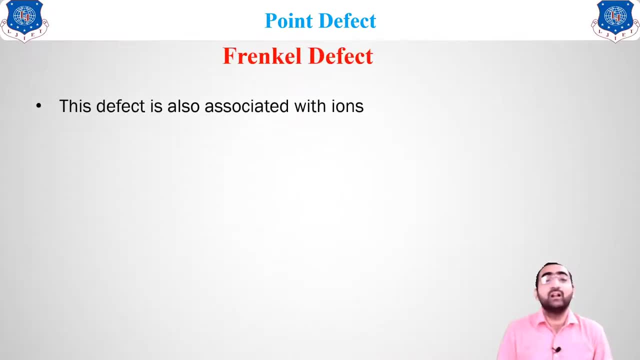 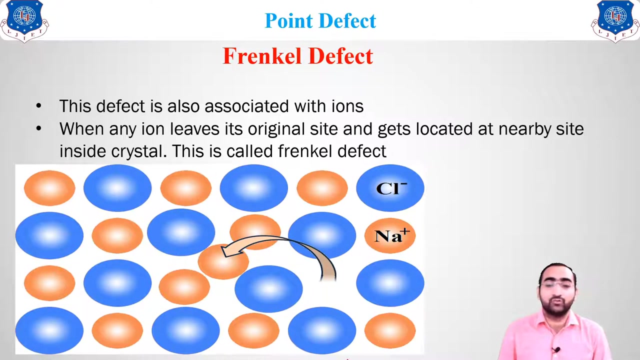 defect there it is known as in Frankel defect. Frankel defect is also associated with ions. when any iron leaves it position, but inside a crystal only, it goes away and settle down, then that type of the thing is known as an Frankel defect. you can see over here the one sodium atom over here is a positive and and non positive. 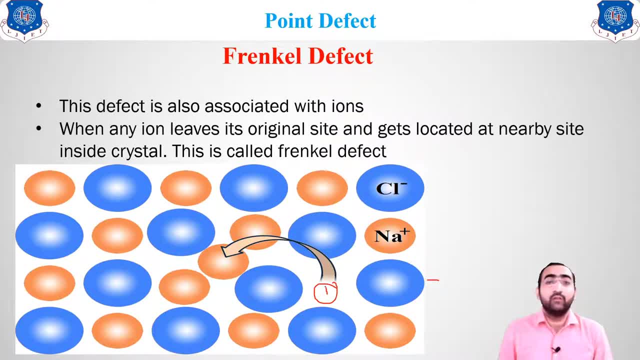 here, one sodium atom is there it it have left his position and just goes away and have settled down at any space in the crystal, only not going outside of the crystal. then that type of the defect is known as an Frankel defect, Short key Frankel. they are the types of the defect occurring due to the 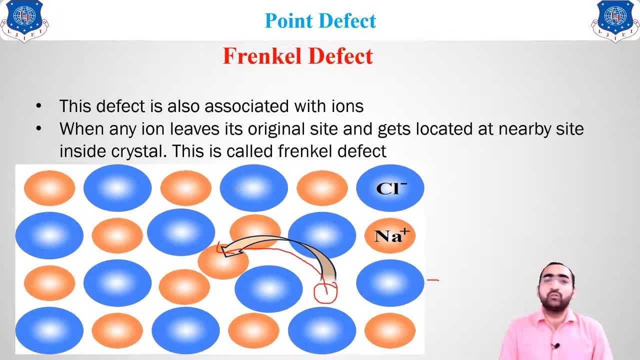 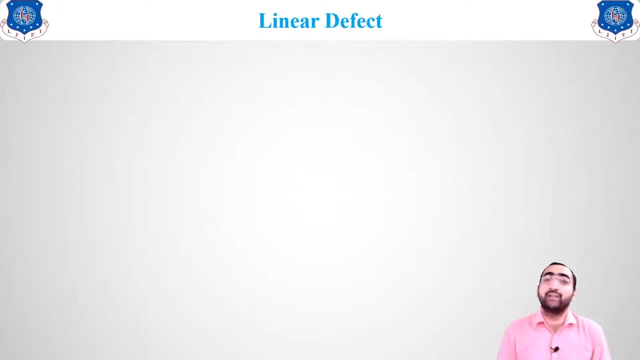 ions clear. So this was about your very first defect, that is known as an point defect. Now moving forward for the linear, or you can say it as a line defect. What do you mean by the linear or the line defect? They are the arising of addition or subtraction or the deletion of a. 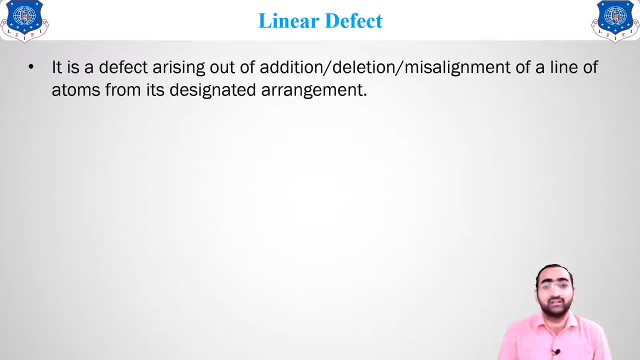 particular whole line of atoms in a crystal. that type of the thing is known as a linear defect. Why does it occur? It also occurs due to the solidification and the plastic deformation of the material. During plastic deformation there is a large movement of atoms due to 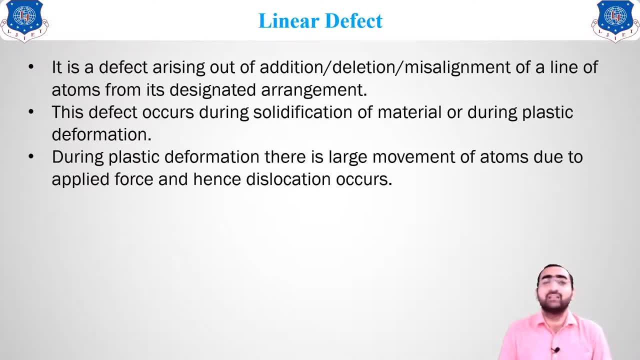 be due to the solidification of the material, So this is known as a point defect. So this is the force applied. So what will happen? There are chances of atoms going away or getting inside a particular crystal and due to that the defect occurs. How many types of the defects are there? 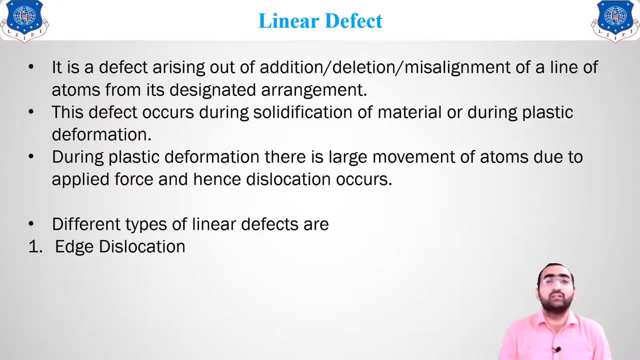 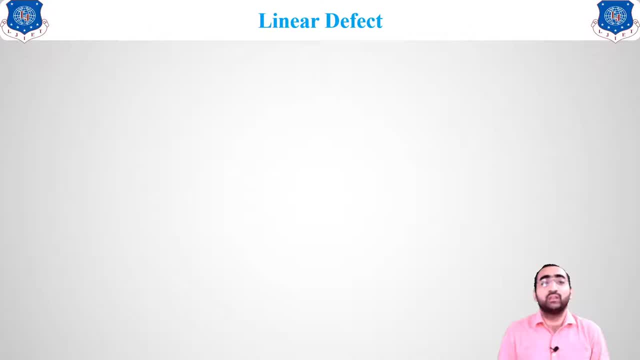 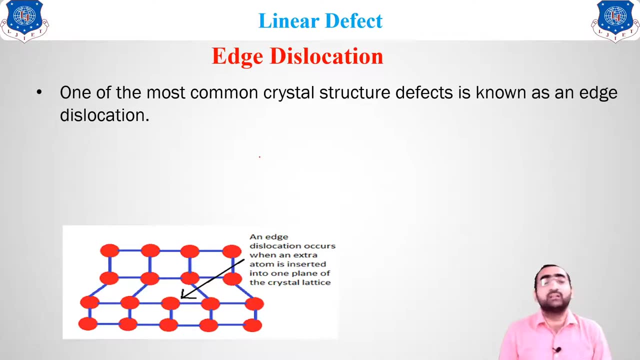 There are two types of the defect which occur. The first one that is known as an edge dislocation. Second one, it is known as a screw dislocation. Now let us discuss this, both the things. First one, edge dislocation. Let us discuss about the edge dislocation, One of the most common crystal defect. 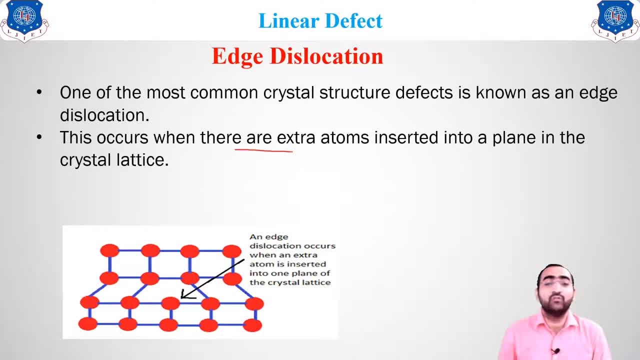 that is known as an edge dislocation. It is occurring due to the extra atom inserted in the crystal structure. You can see over here these two atoms, that is, an extra atom, which are there inside the crystal. What will happen? Edge dislocation make it easier for atom to slip. 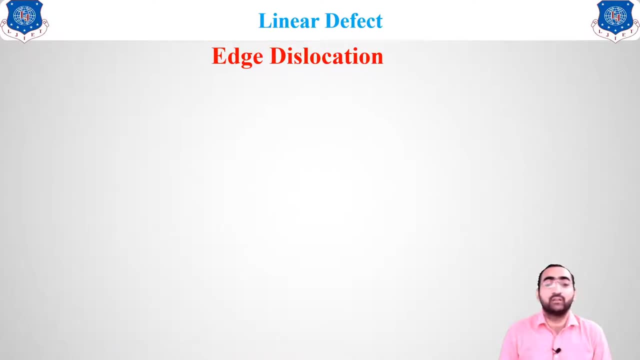 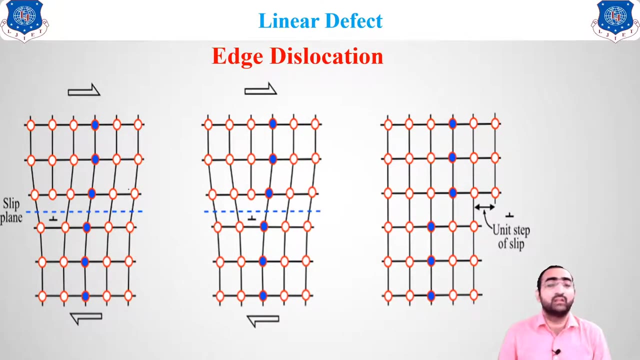 Now this thing will slip over the surface and, as a result, you can see over here. see, this is the surface in which there is a blue color thing. that is all this thing. This is the atoms, which more are coming inside the material. This line is coming inside the. 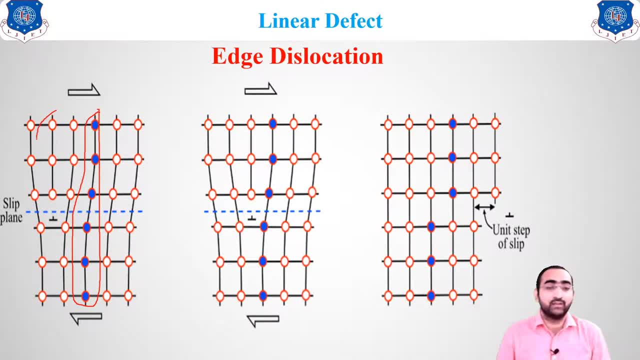 material. So over here there is a force and you can see over here these three atoms. they are the addition. Due to this, the force is applied. What will happen? This atom will proceed further. So you can see over here, they have reached over here and, as a result, it will move away and it will 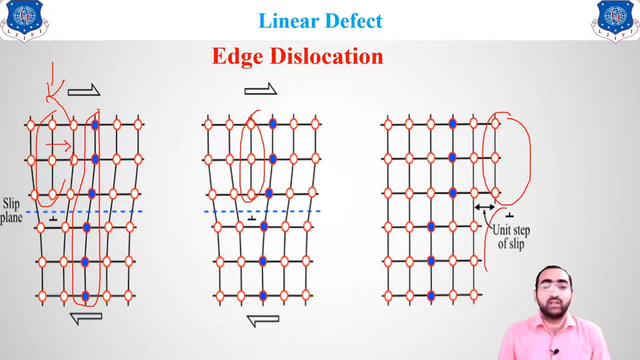 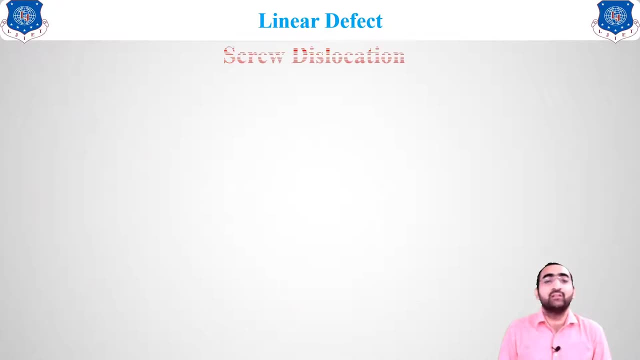 reach over here and, as a result, you can see there is none of the atoms lying over here and this has slipped. So, as I told you in the previous slide that the material will try to slip on the thing. So that is the thing, how edge dislocation occurs. The second one that is known as an screw. 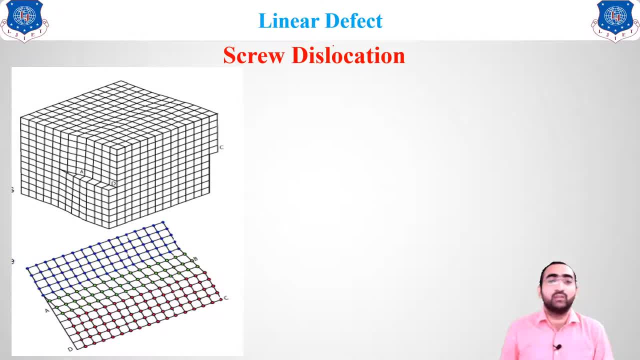 dislocation. Screw dislocation is this type of the thing in which you can go for the particular, this type of the defect. Screw dislocation is this type of the thing. and edge dislocation is this type of the slipping of the material, When you take a material and just goes away for the 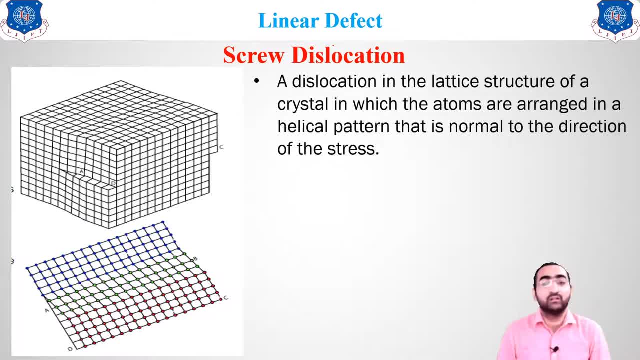 torsional force, then you can see that the material is slipping. So, as I told you in the previous slide, that the material is slipping. So, as I told you in the previous slide, force, then the screw dislocation occurs. It is the latest structure in the crystal in which 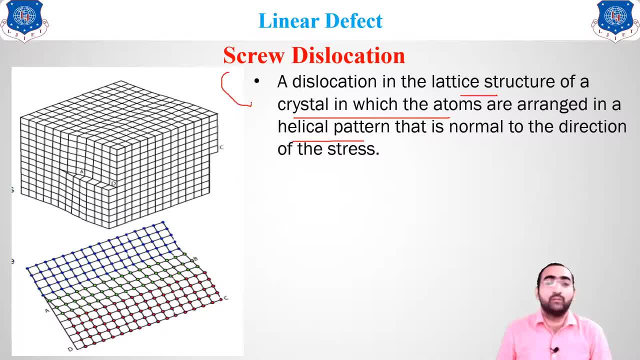 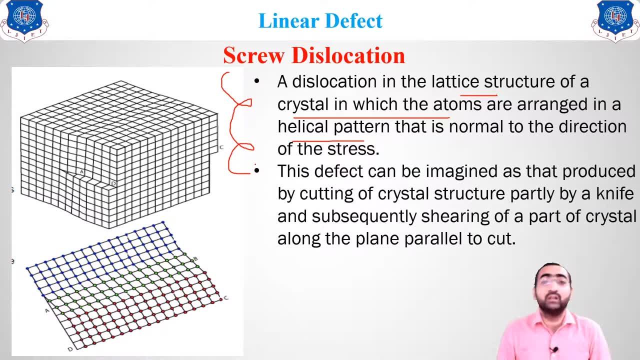 atoms are arranged in a helical pattern. Helical pattern means they will follow this particular helical pattern. when a normal stress is given, The defect can be imagined. Imagine a defect in a closed book. If you take a knife and insert that knife inside a book, what will happen? You can see. 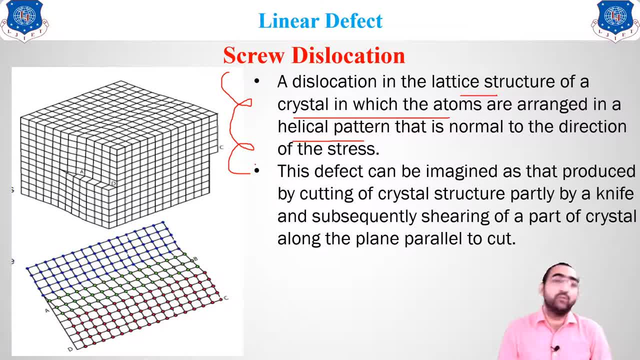 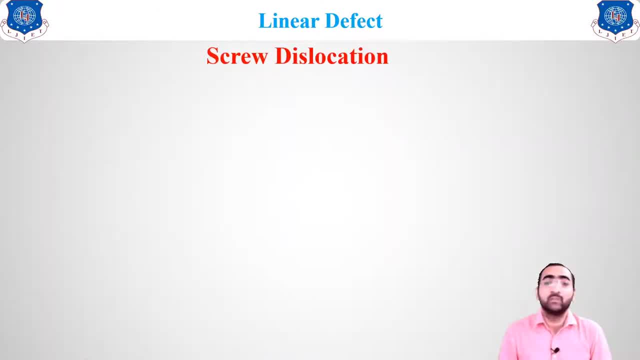 that there is a bulging coming out of that book. Why? Because a knife is there inside a particular book. So that is how your any of the screw dislocation occurs. Now let us see how the screw dislocation takes place. Over here you can see there is a turning force which is applied due to 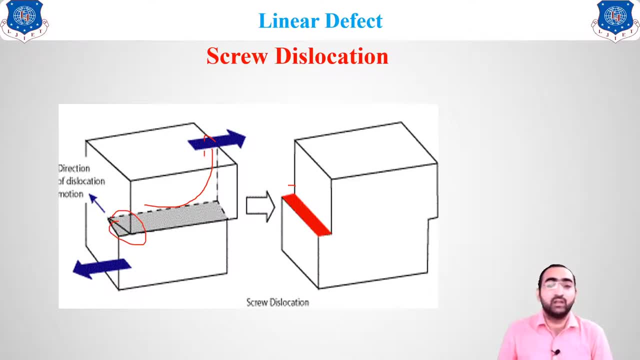 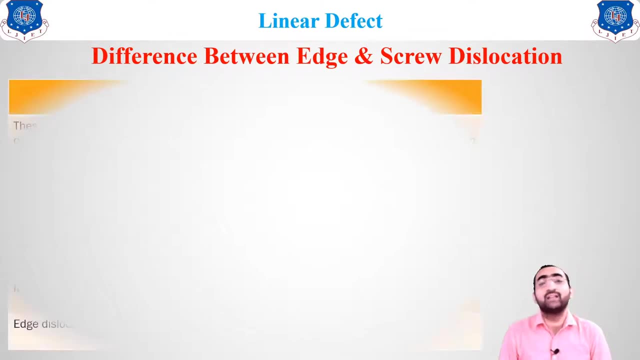 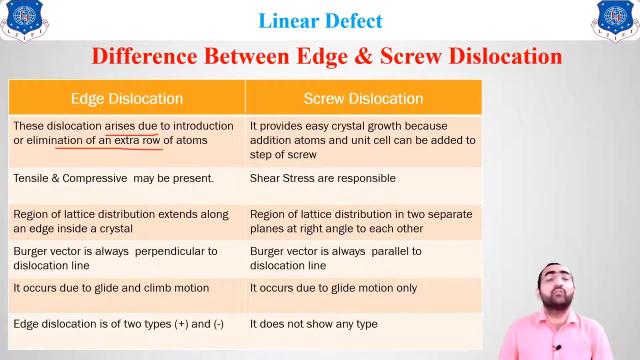 which it will slip on the atom. This is the thing how it appears, due to the screw dislocation. So now let us discuss what is the difference between edge and screw dislocation. The dislocation arises due to introduction or elimination of extra row. Here it is the crystal growth between because of the addition of the atom. That means 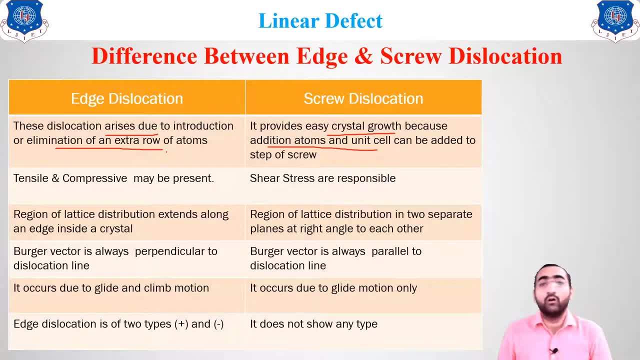 over here either the atoms are added or removed. Over here, only atoms are added in a line. Tensile compressive load must be present Here. shear stress. they are responsible. Region of latest distribution exceeds along the edges. only Over here it will move in the right. 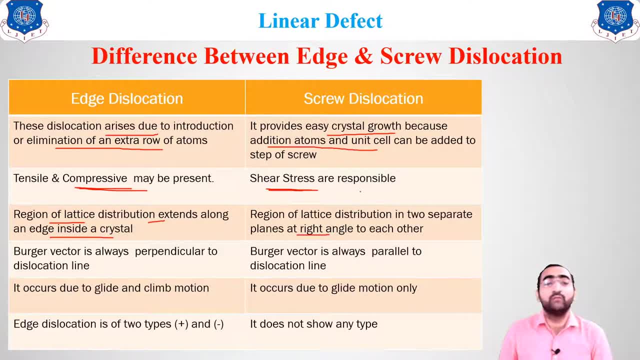 angle. It will proceed further. That means it will move in the right angle. It will proceed further In the upper direction. That means two separate planes at 90 degree. we will be getting Berger vector. there is one imaginary vector. They are always perpendicular to the dislocation line. 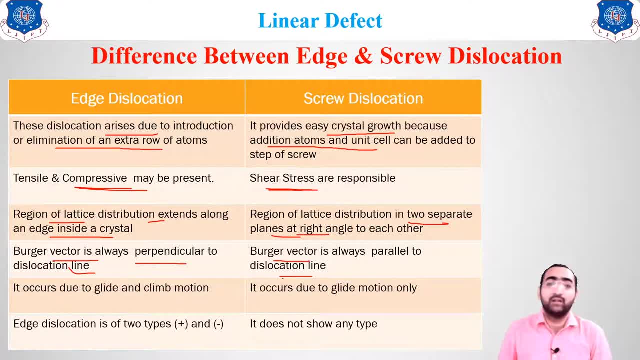 Here berger vector is always parallel to the line. That means a dislocation line. It occurs due to glide and climb, But it occurs only due to glide motion. There are two types: positive edge or negative edge. Introduction: they are of plus sign. and elimination of the atoms: they are of the. 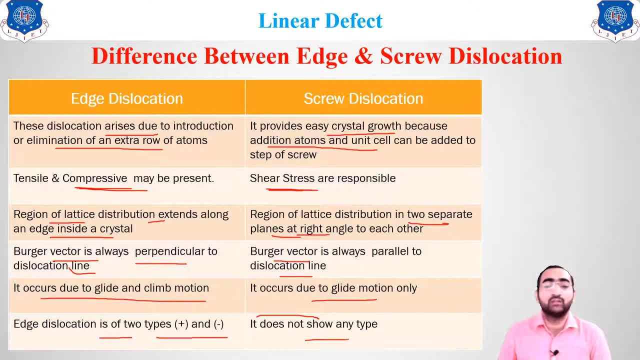 negative edge dislocation. There is no type which is there in this screw dislocation. Clear, This was all about your line defect or you can say linear defect, in which we have studied two types of the defect, that is, edge dislocation and screw dislocation, Moving forward for the surface defect, the third defect, The 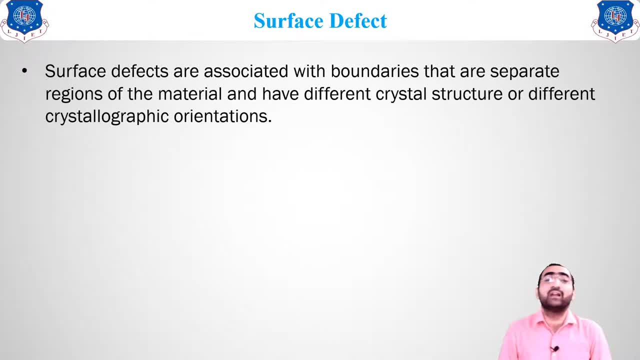 surface defect. they are associated with the boundaries that are separated regions of the material and due to which the crystal orientations has been changed. Now this defect is not a defect. It is also caused by the solidification and due to the heat treatment which we are applying. 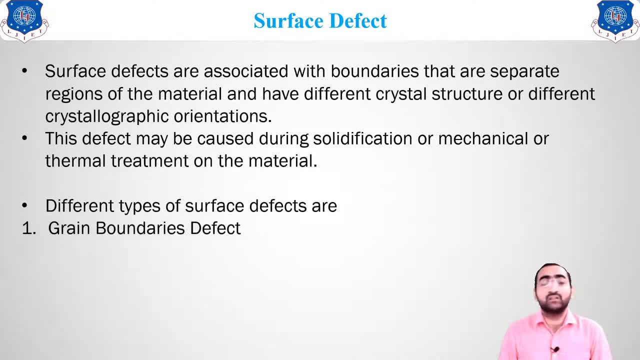 on the material. Now, there are different types of the surface defect. They are grain boundary defect, tween boundary, tilt, boundary, stacking fault. These are the defects which are occurring in the surface defect. Let us discuss about the grain boundary defect. You can. you might be knowing about the 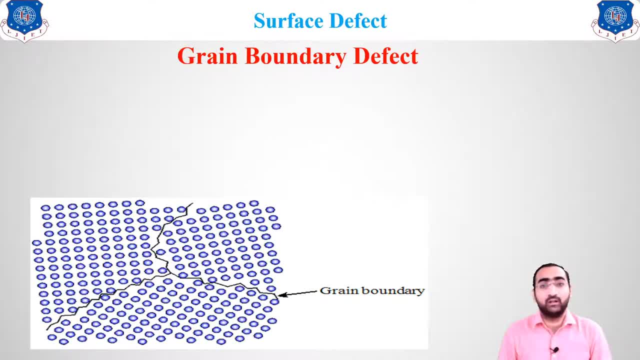 grain boundaries. What do you mean by grain boundaries? in a material, the different types of the crystal they are having, the atoms are arranged in a different way. So in a material, the atoms are arranged in a different way. These atoms, they are the one colony. These atoms, they are the another. 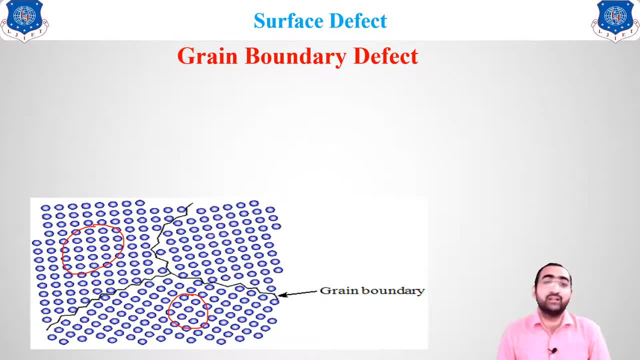 colony. The sitting arrangement: they are different As the students are sitting in the different classrooms in the different pattern and that two classrooms are separated by a wall. In the same way, the two crystal phases: they are separated by the grain boundary. These are the grain boundaries. 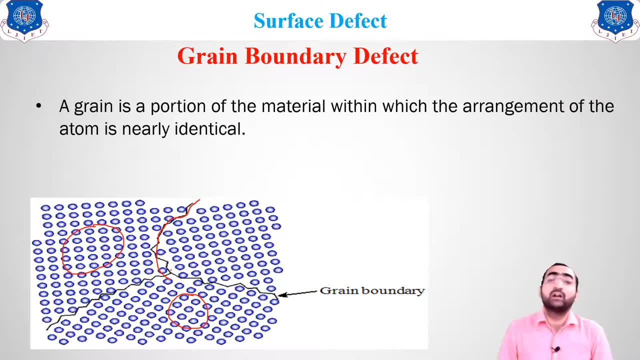 and due to that there is a defect which is occurring. A grain is a portion of the material which are arrangement of the atom nearly identical. That means they are not separate out. the two different types of the Mukbang Bobby defect are cause due to the separation of the grain and the different orientation for the polycrystalline material. That 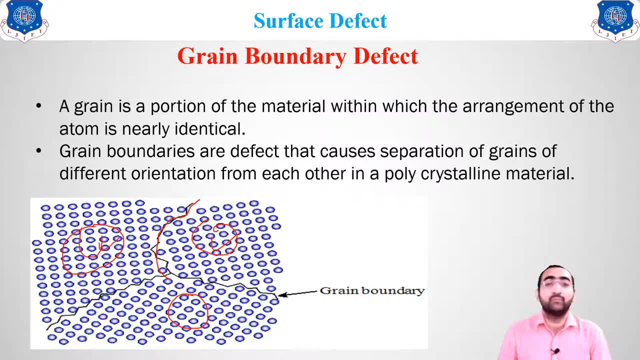 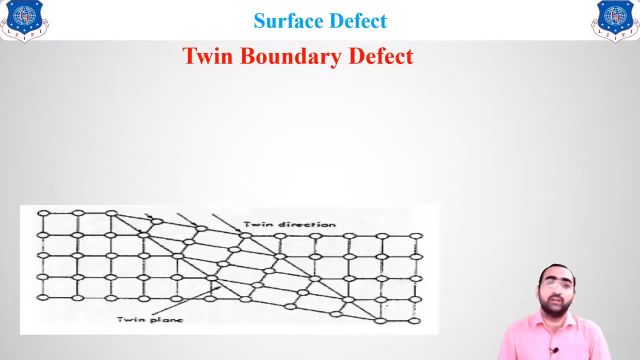 means the sitting arrangement of this is different and this is different. That means the same way. there is a tollars. today We're in the boundary, the exit we need winning. that means the duplicate dangling之後. due to that, there is a twin surface defect, is there? what do you mean by this twin boundary? 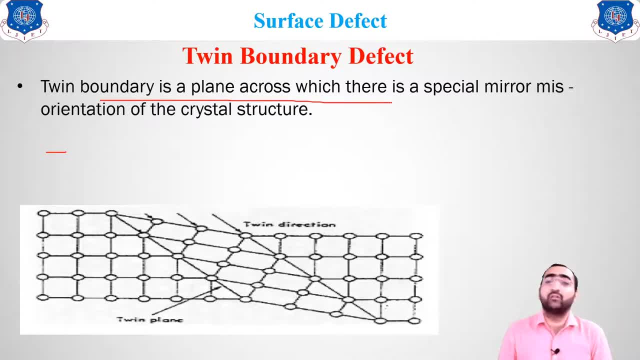 that is, the twin boundary is a plane across which a special mirror misorientation of the crystal structure is there. the region of the material between these is termed as a twin. you can see, it was the thing that is. it was a straight line. it was a straight this. all the atoms are where. 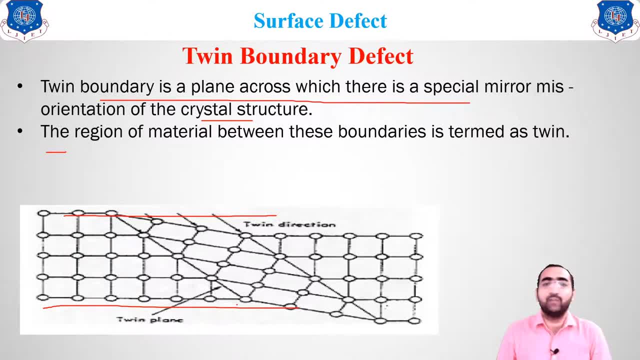 in the same plane. but what happened? due to certain type of the force or the heat treatment, you can see this type, this thing. they have slightly changed that orientation and have slightly came down. so this region is known as an twin plane by where it has gone for the translational thing. 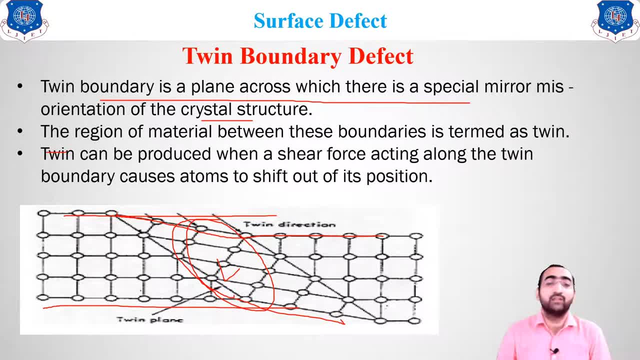 that means slanting thing, whatever thing they are there. that is known as an twinning effect. twin can be produced when a shear force along the twin boundary causes atom to shift out it position. so the shifting of the whole surface over here, if there is a surface, is there and due to certain 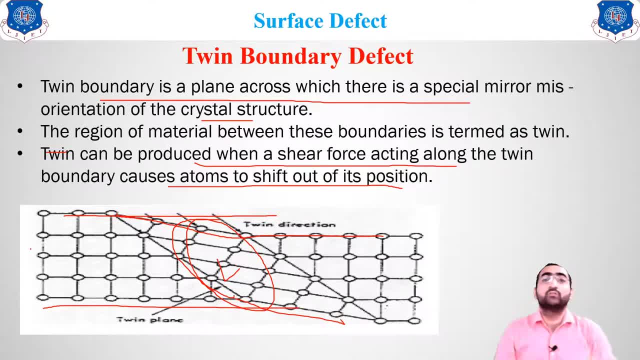 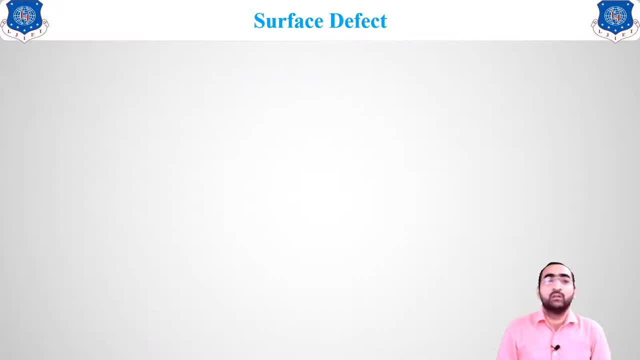 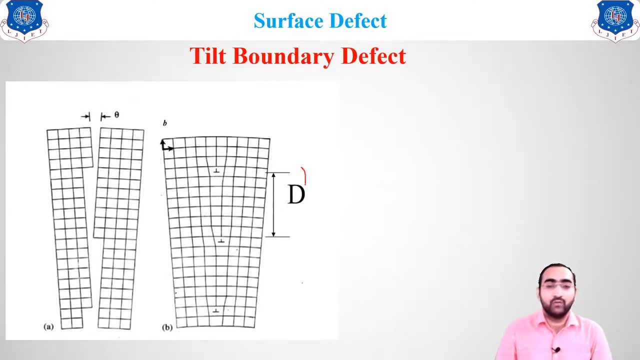 force if this thing has come down and gone away. so that is how the twin boundary, due to certain force applied on the surface, the twin boundary defect occurs. the next one, that is the tilt boundary. when your particular material, the boundaries are tilt, if in a thing, if you are 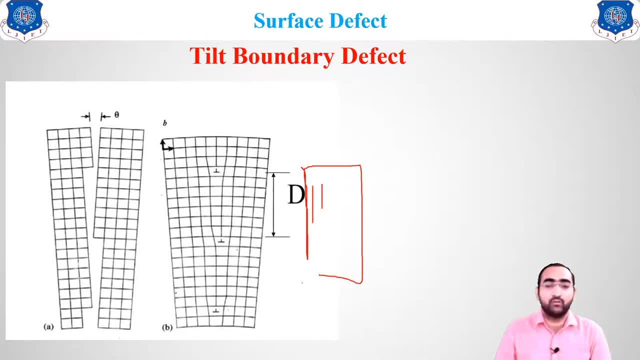 having a structure in which all the atoms, they are located in a straight line and if, due to any reason, there are changes in the small angle you can see over here, the small angle changes you can see in these boundaries, then that is known as an tilt boundary defect. small angle grain boundaries. 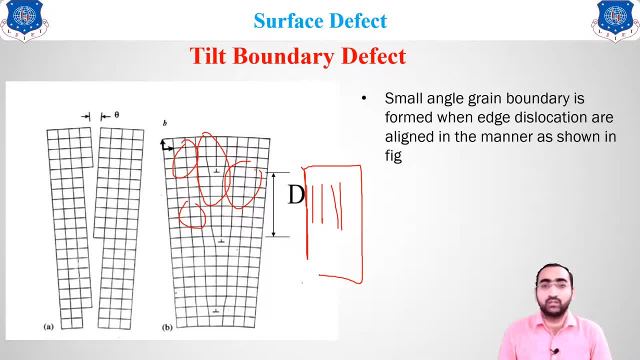 is formed when edge dislocation, due to edge dislocation, this type of the tilt boundary that means original, it is like this, but due to the thing edge dislocation, it has slightly changes orientation by certain small angle tilt boundary between the two slight misalignment appear as an area of the edge dislocation and as a result it appears as a defect and the 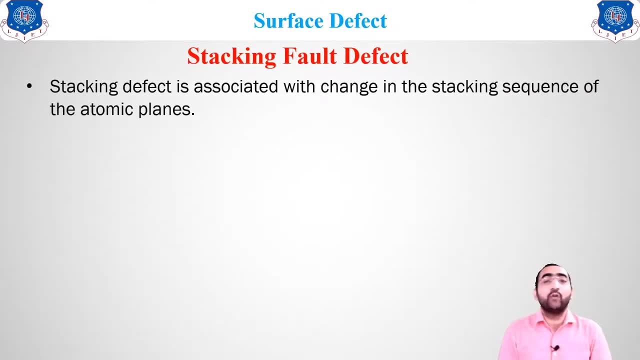 last one that is known as an stacking fault defect. stacking fault, they are basically the thing or the stacks, how the atomic planes are arranged. it is on that if an original thing of stack that is abc, abc type and, due to certain reason, reason if there is a change in this stack. 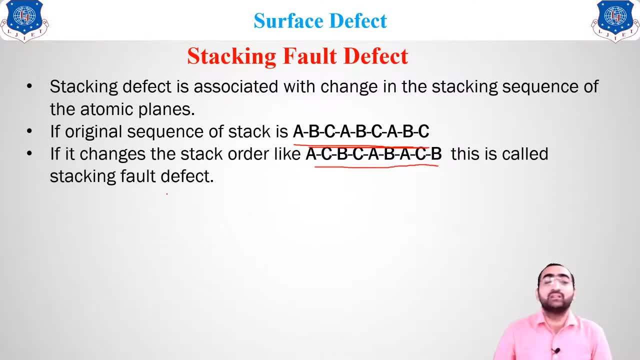 that means ac, bc, ab, acb. this is a stacking fault. means there should be always a, b, c, a, b, c is there, but due to something, if the thing that is a, c, a, b, this type of the stack means layer by layer, if from the original they are been getting. 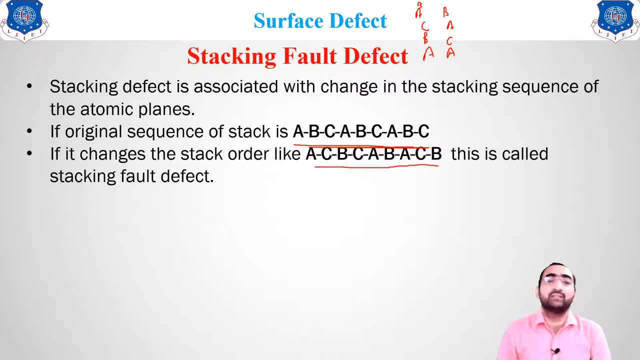 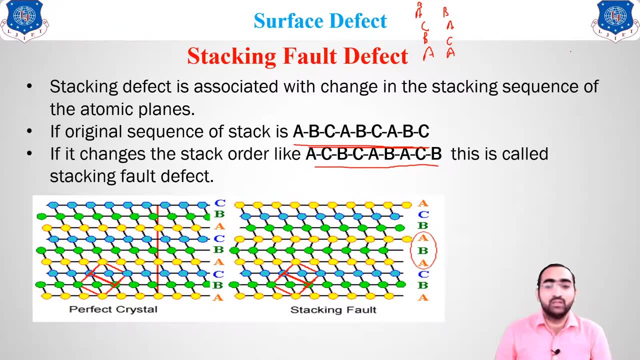 changed, then that type of the defect is known as an stacking fault defect layer. so this is how you can see over here the abc, abc type is there and they have been replaced by the thing that is the stacking fault. so here you can see abc, abc type of crystal and here the there is a change in the.